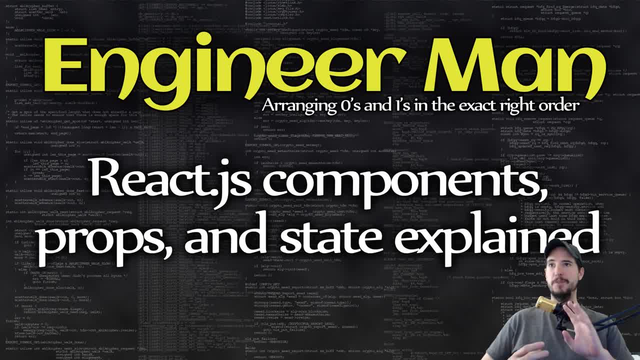 What's going on, engineers? I'm back with another React video and in this one we're talking specifically about components, props and state. Prior to this, I did a getting started with React video. If you're new to React, you should definitely watch that video first. I'll 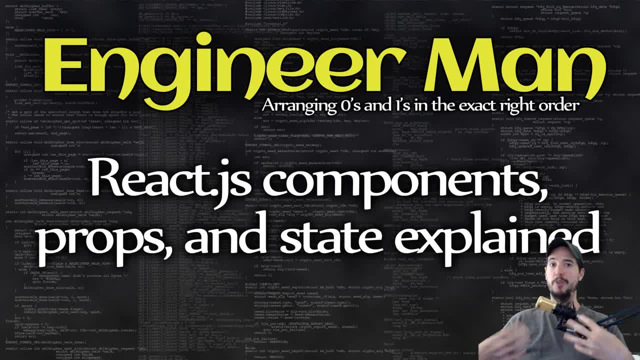 link it in the description, because this video assumes that you at least know how to create a component. If you already know about React and you just want to learn more about components, props and state, then you could probably skip that video and just keep watching. 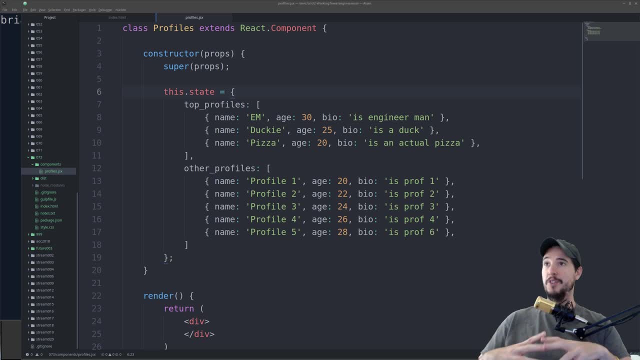 So we got lots of cover, so let's just jump in. So the purpose of these examples is to show you how you can take larger components and break them down into a couple smaller child components which you can include in your parent component, And once you've done that, we can use this thing. 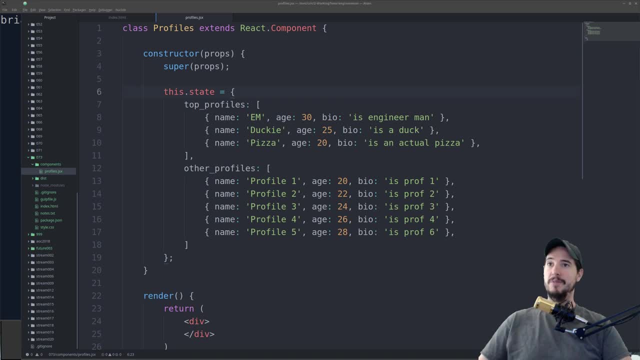 called props to push data down to child components, And what we're building today is a profile lister. so we'll display a heading called top profiles and it will display stuff from thisstatetop profiles and it will show a heading called other profiles and then display the other profiles. 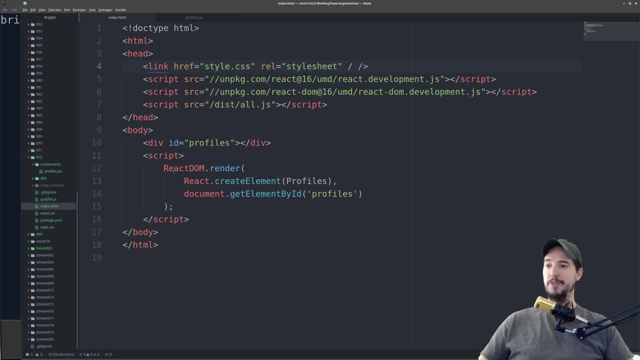 under that And I'll just quickly show you what the HTML looks like here. I'm just using reactdomrender, I'm creating an element called profiles, and then I'll just show you what the HTML looks like here, And I'm inserting it into the profiles div And from here the video. we're not going to need to. 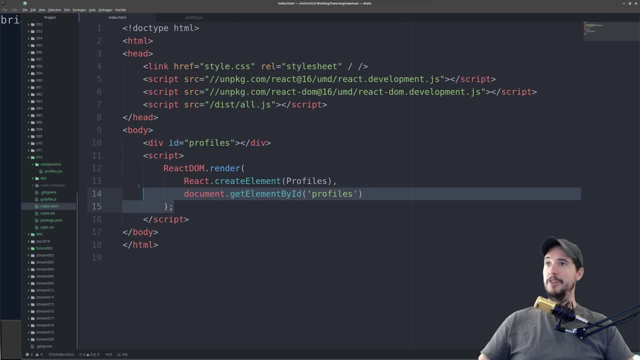 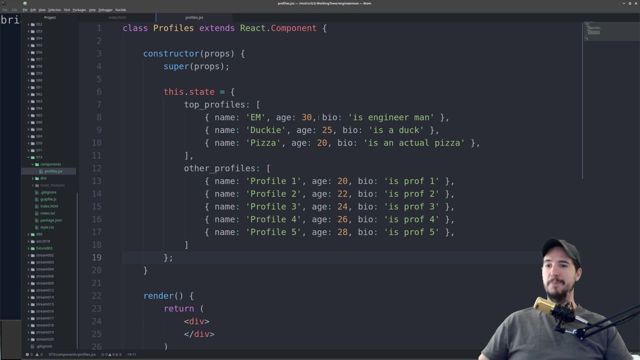 touch this. This can just stay as is for the entire time. If you're not sure what this does, definitely just pause here and check out that first video that's linked in the description. So we have some profile data here, like name, age and bio, like EM, age, 30, bio is engineer man. 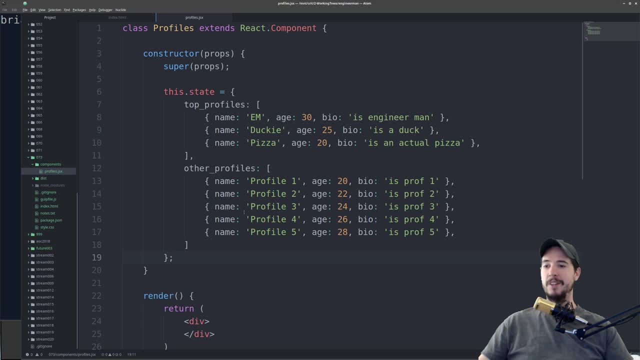 got. ducky is a duck and pizza is an actual pizza. Then we have some other profiles here, one through five, and then bio is prof, one through five, Simple stuff. So now we're trying to build the UI and all we're going to do for the UI is: we're going to build the UI and we're going to 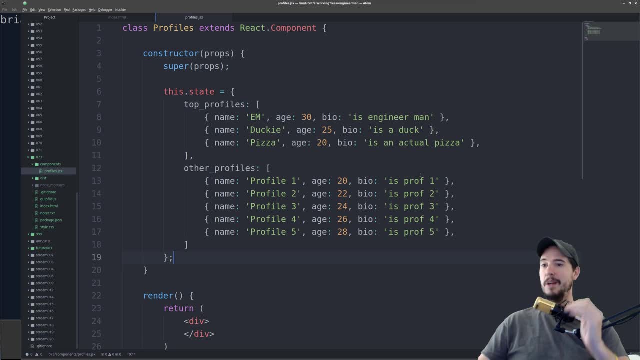 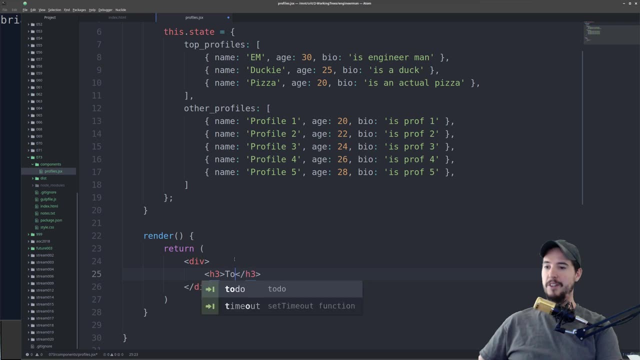 have an image and then to the left of the image is going to be the name of the person and then the age and the bio. That's it, real simple. So we'll start building that UI up. First thing we got to do is just do a header. So we'll do, like you know, top profiles And then under 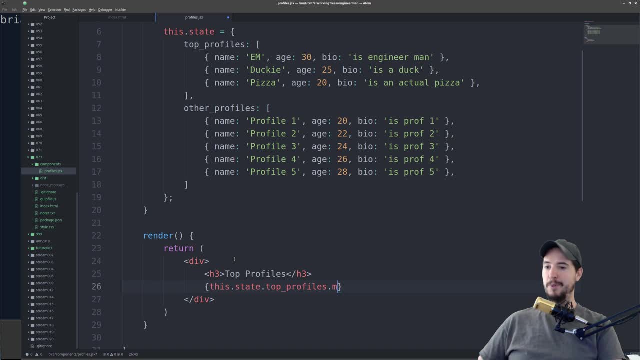 the top profiles. we want to loop over everything in the top profile, So top profilesmap, profile, and then here we could start typing the HTML for the profile. So we'll put a new div to put the profile in. We'll insert the image. Next we'll drop the person's name in there with an h4,. 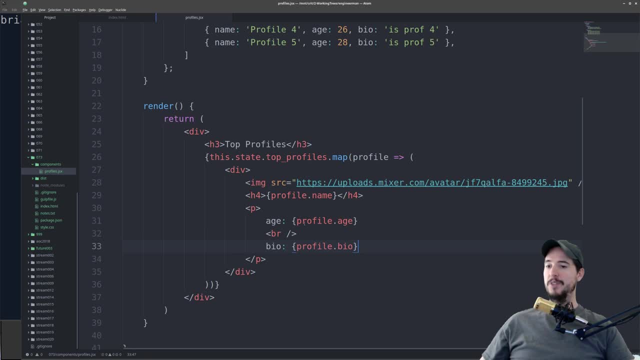 create a new paragraph And inside there we'll drop the person's age and bio. So at this point we should be able to come over here to Brave, hit the refresh button and we should get something. So our UI is good. It shows. 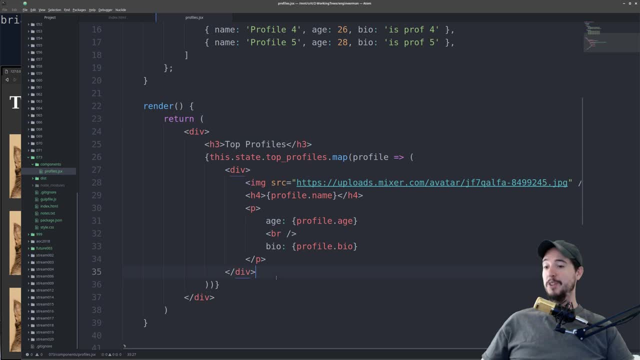 us our top profiles. Everything's good to go so far. So next thing we got to do is show the other profiles. So we make a new header called h3, other profiles, and then we copy and paste all this code here. Well, no, of course not, because we're good engineers and that's ridiculous. 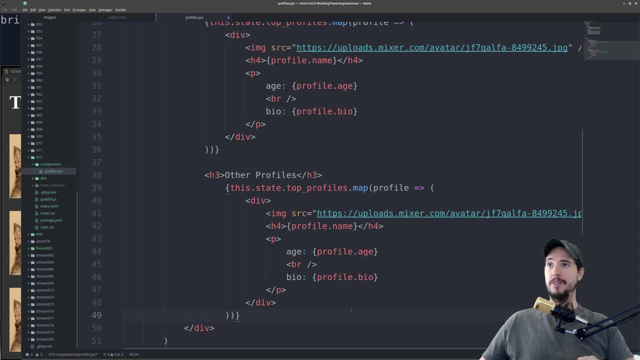 So how can we save ourselves from the ridiculousness of tons of code? Well, you'll probably be unsurprised to learn that the answer is child components. So to create a child component, and since we're doing profiles as the parent component, it would make. 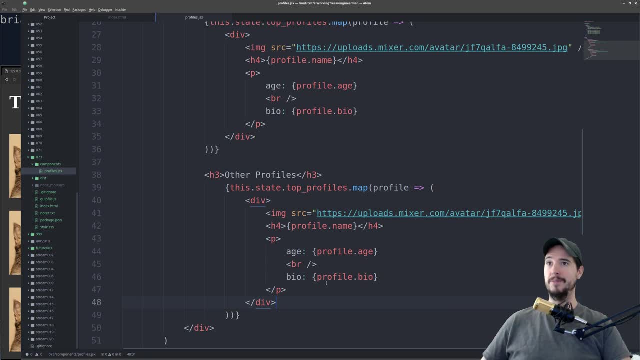 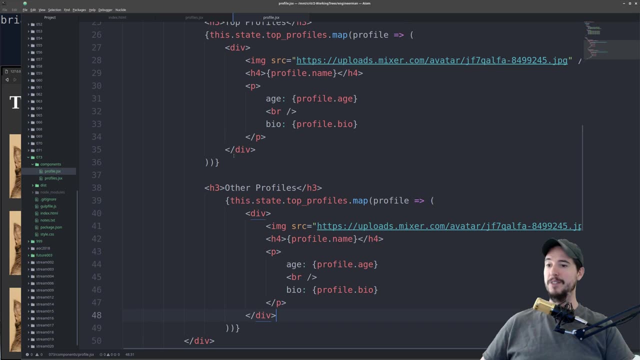 sense if we would create a child component called a profile singular. So let's start by just duplicating this component from profiles to profile. So now I have an exact copy of profiles. All I really need to render here is just the one profile, So I'll copy just the profile portion of. 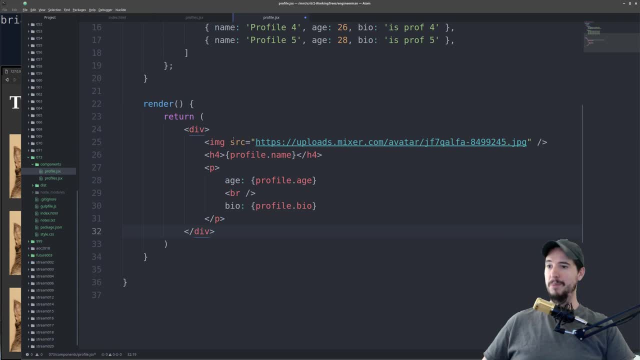 this, And then I will get rid of all this other HTML And just leave that. And because this profile has no state, which is to say that I don't need to actually modify anything about the profile after I render it, I can actually just remove this entire. 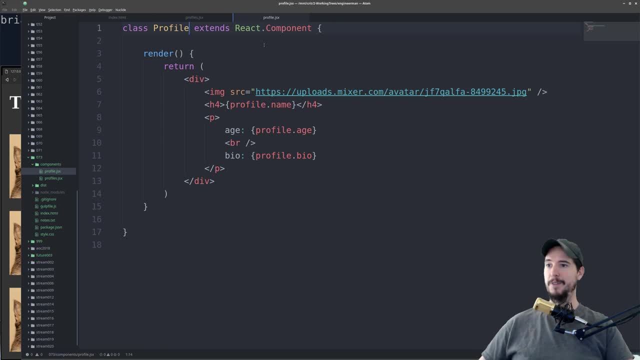 constructor entirely. just get rid of it And I'll drop the s off of there. So now it's profile. So now I have a component called profile And all it does is render the HTML that came from the profiles component. So I have to change. now is this: profile object doesn't exist And this: 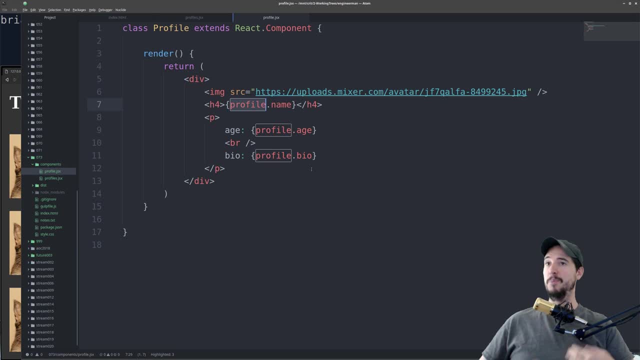 is kind of where props comes in, because what we're going to do is we're going to pass the profile in to this component and we can use it here. So what we'll need to change this to instead of profile, it's going to be this: dot props, dot profile, And this will make more sense in a second. 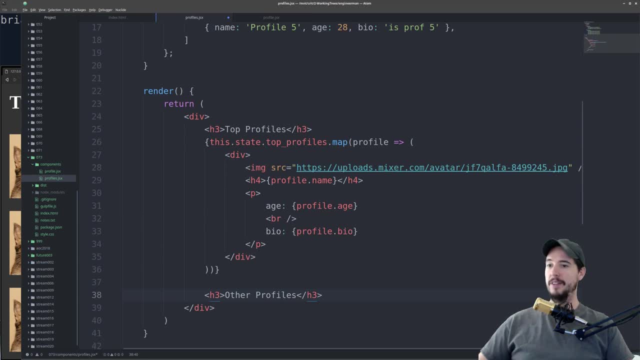 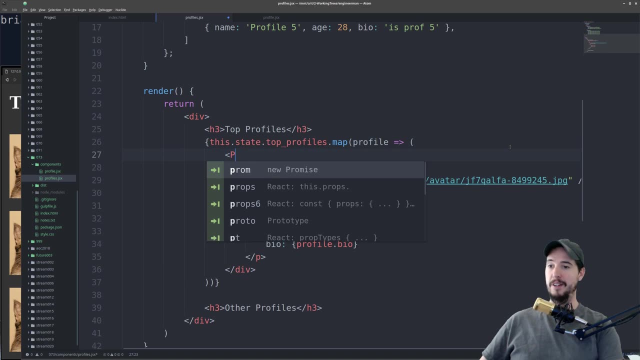 So we'll start by deleting this block. we don't need it just now. And then the way we're going to convert this to use the actual profile component is, rather than supplying all this data, we're going to supply profile, And that will create a new component in that place. Now here's where. 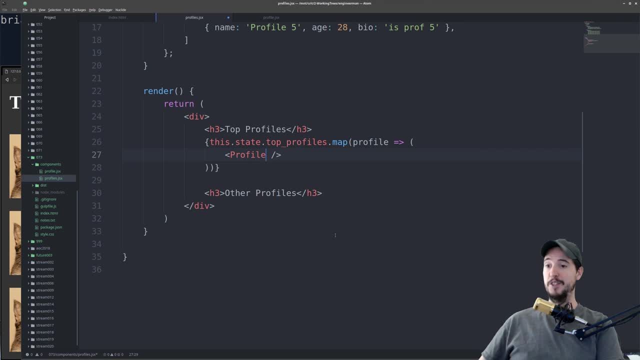 props comes in. If I want to pass something to this component, I can specify it in the HTML attribute So I can do. profile equals this sorry profile. So anything that supplies an attribute here goes into this dot props of the component. So now when I come back to profile, 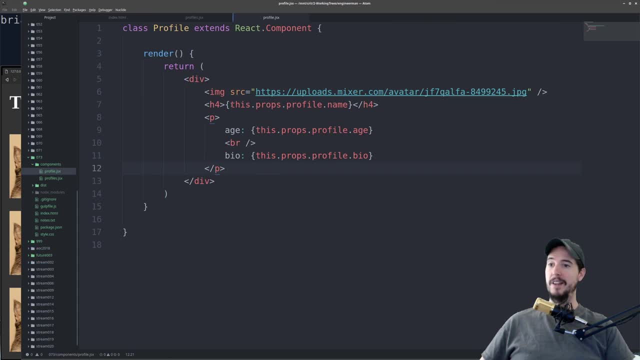 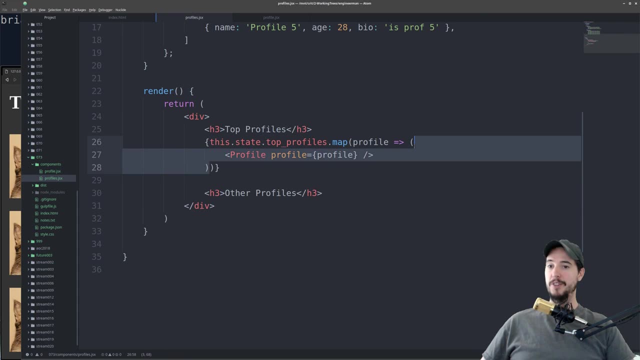 I have access to this dot props dot profile And that's why I can render now name, age and bio And I don't even need these this parentheses anymore. I can actually just take this and I can just paste it in place of here, And that will work just great. So real quick, I'll check in. 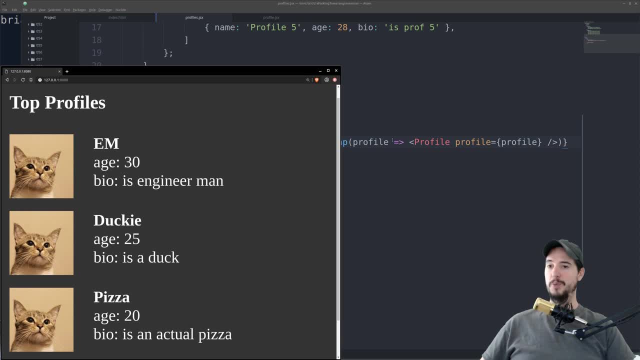 brave, just to make sure that I have all the data in there And then I can just paste it in here. Nothing's changed. I hit refresh and everything looks fine. So everything's working. it's rendering those child components correctly, So now we can finally render the other profiles. And now we just 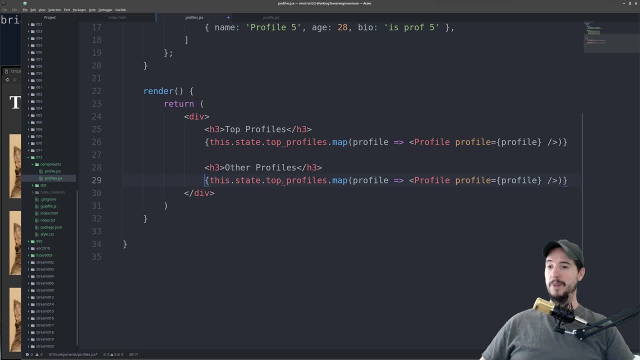 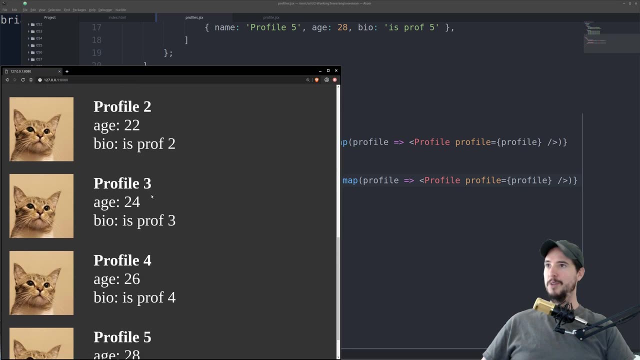 copy the one line, which is no big deal, And then replace top profiles with other profiles. we can come back to our browser, hit the refresh button And now we have a bunch of other profiles that show up And everything seems to be working fine. Now you can create any any amount of nested. 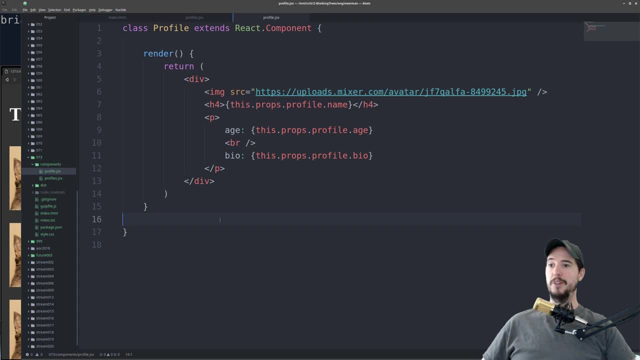 components And you just deem based on what you need in your project when you want to do that And how granular you get is sort of a judgment call. Generally, what I do is when I start duplicating HTML, I know it's time to make a component. I also know that if I am going to 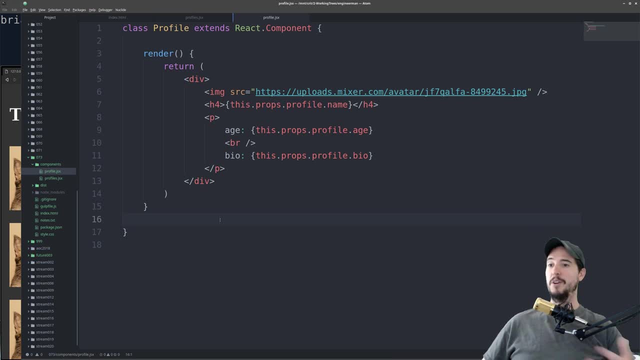 make a component and it'll end up getting used in 10 spots, then I know I should probably make a component versus putting the HTML in every component. So, just for fun, we're going to create a new component called name, which will just be the contents of this h4 tag. So I'll create a new. 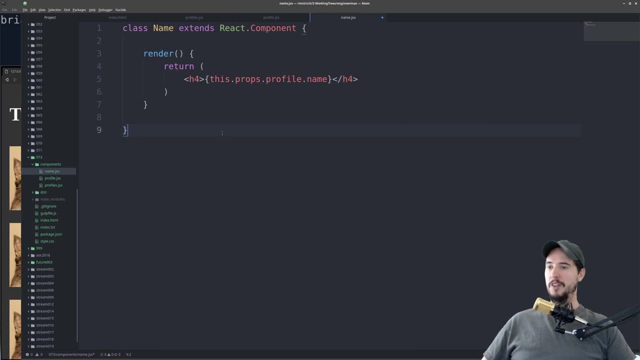 component called name dot JSX. I'll drop that in there. this dot props dot profile dot name, except this one will be modified slightly. I won't do this dot props dot profile dot name. I'll take out the profile. So it'll just be this dot props dot name And that way. 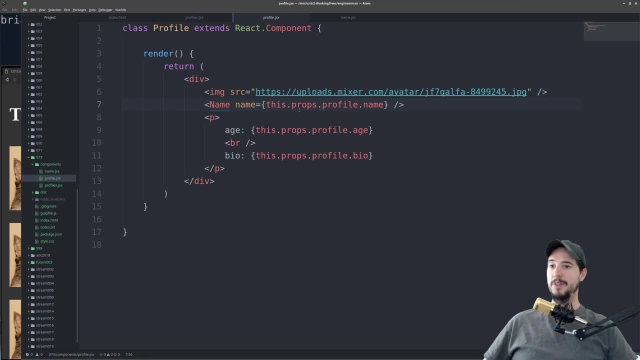 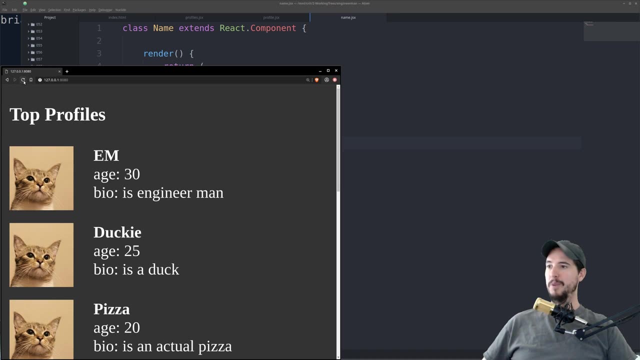 when I come back to profile I can replace this with name. name equals this: dot props, dot profile, dot name. That way I can just use the prop called name And that's it. And again we'll come back to brave. just to refresh, just make sure everything's okay And it is working. fine, name is still there. 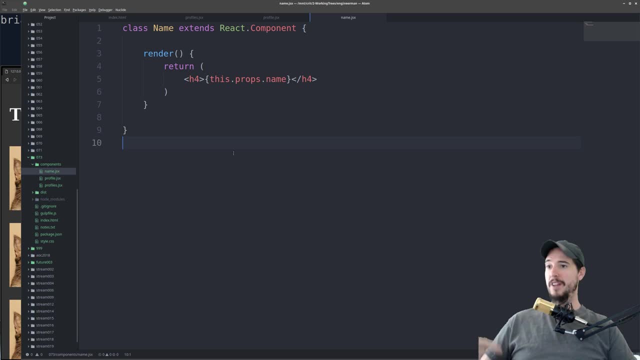 Now the last thing I do is simplify this a couple times, because this doesn't have any state and only use props. you can actually do this, So I'm going to do this, And I'm going to do this And create what's called a stateless component. So what I can do now is I can take this return. 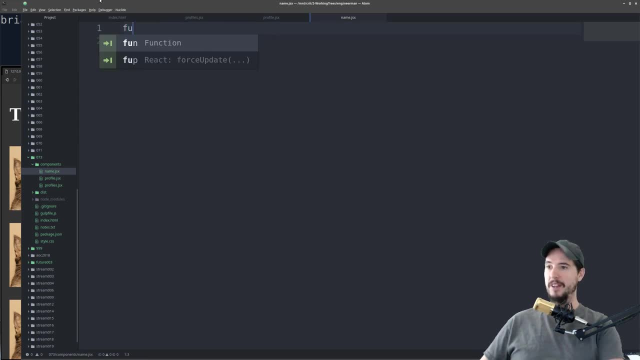 statement And instead of using class, extend, react component and this, and that all I have to do is do function name, throw props in there and specify return. I then just have to just drop off this And then now it's just props dot name. I can come over to brave, hit the refresh button. 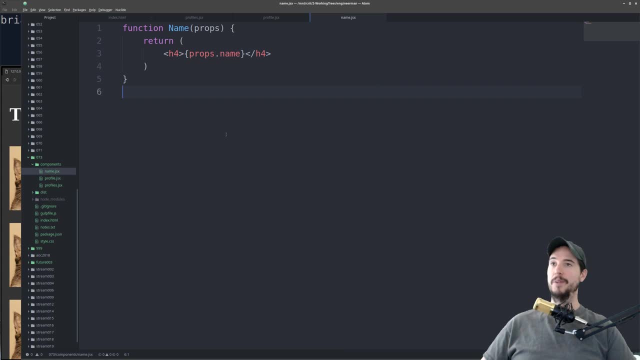 you can see that it still works fine. Now I have a really, really simple component. I can even make this even simpler. If you can even believe that you can do something like const name equals prop and just do it this way. This would be using an anonymous function versus a normal function, So 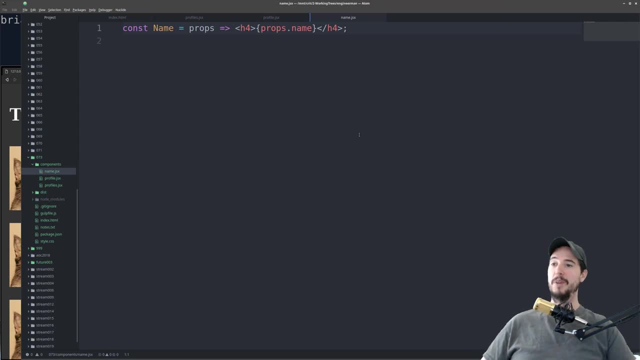 this is about the simplest possible react component you can make, But you can see that you come back here and you hit refresh And it still works. It's fine. This is still a legitimate component. The last thing I want to talk about is state versus props. I get asked a lot like: when should 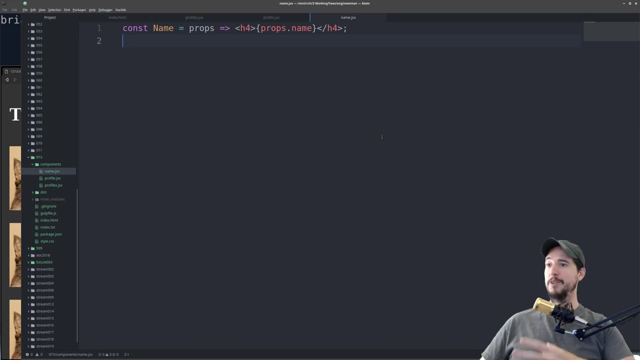 I use state and when should I use props? Of course props have to be used to pass things down from parent components to child components. So here you have to use props- profile equals profile, and then profile you have to get access to that via props. So in that, 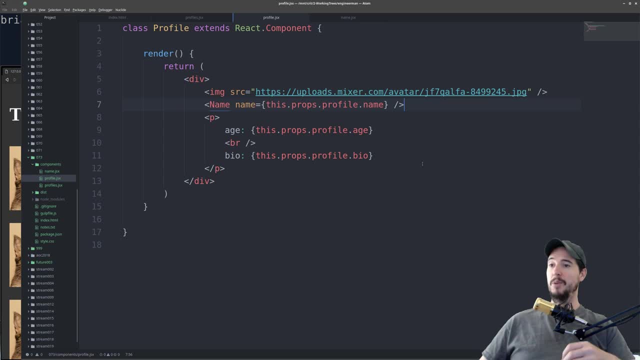 case, props is essential, But there's a second part of it, And it's when I render HTML in a component. should I use props or state? And the answer is: you can use props if the data cannot be changed by a component in that UI. Otherwise, you should use state If you do know that something. 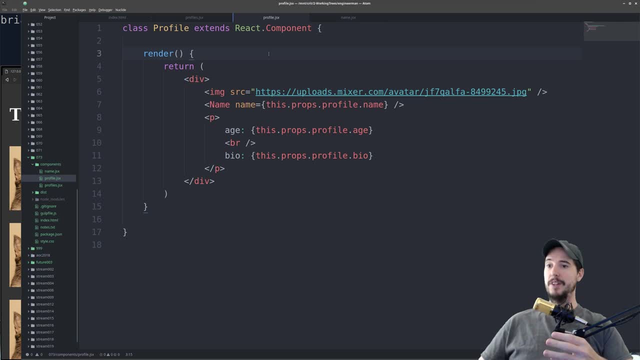 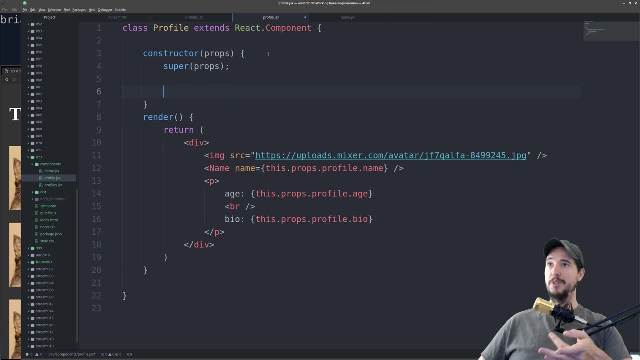 for instance, in the profile component can say change the age, then a common pattern you would do is you have to reintroduce the controller, the constructor, of course, and then what you would start out with is you would create the initial state. 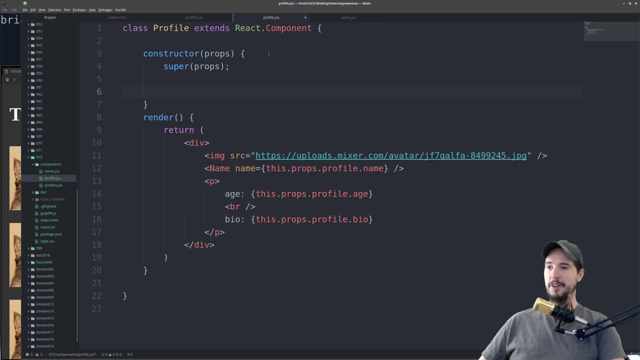 and then you would apply the props to that state. So here you would set initial state: this dot state equals, and then you would do age props, dot profile, dot age. Then down here, instead of doing this dot props, dot profile, dot age, you would just do this dot state, dot age. 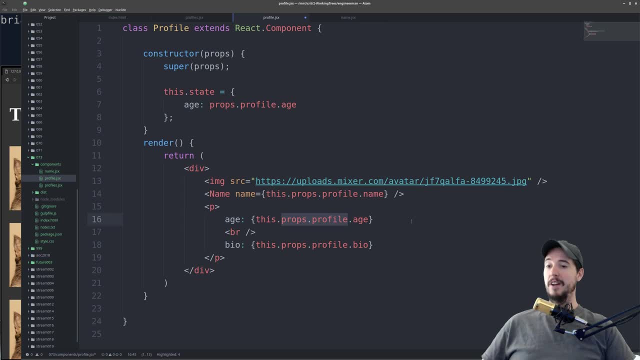 Now, if you expect to modify all of the profile data, rather than setting age is props dot profile dot age, you could just set the entire this dot state dot profile to be props dot profile. Now you've effectively transferred the entire object into the state.